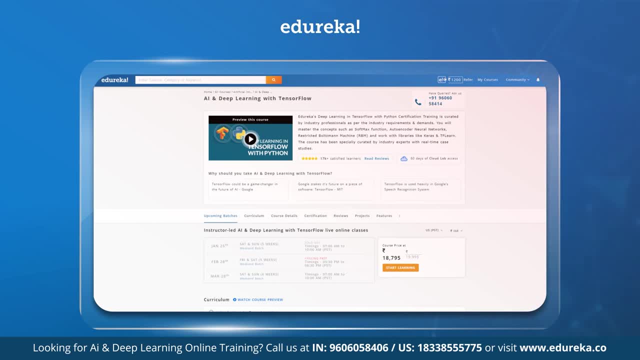 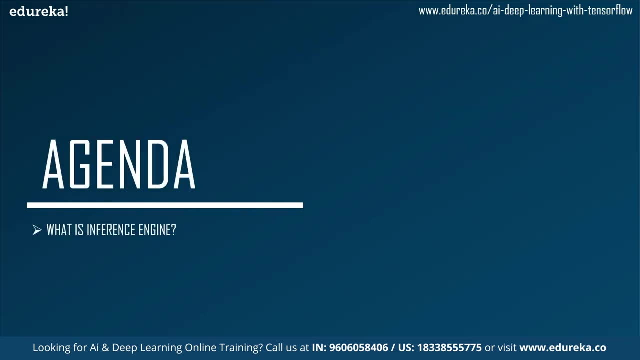 are interested in them, you can click on the link given in the description below. Now let us start this video by seeing what the agenda is. First, we will see what an inference engine is. Now you might ask, Elton, why are you teaching me this in forwards and backwards? 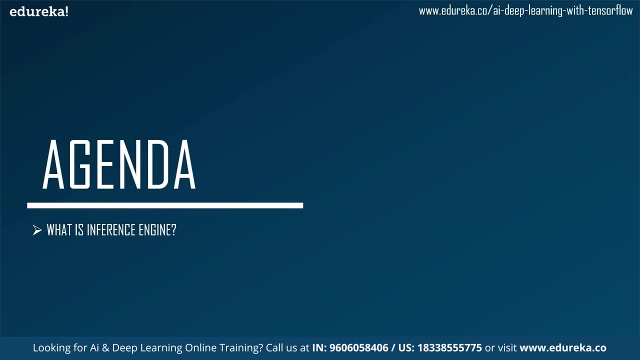 chaining, But this is an essential concept that you need to understand before moving on to the chaining concepts. After this, I will give you an introduction to forwards chaining. What is it and where do you use it? After that, we can see backwards chaining. How exactly is it different from? 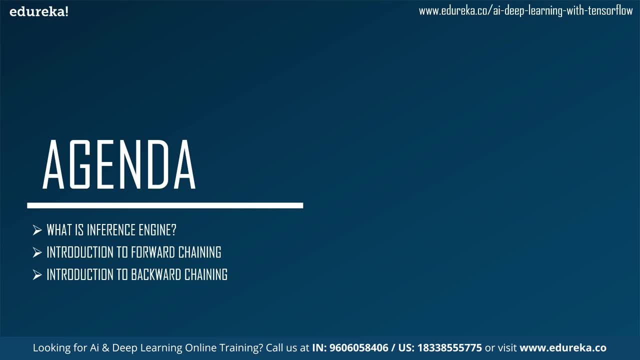 forwards chaining and where can you use it. These concepts will be covered over here. We will end this video by seeing an example. How do you solve this with forwards chaining and how does it differ from backwards chaining? This will give you an in-depth understanding. 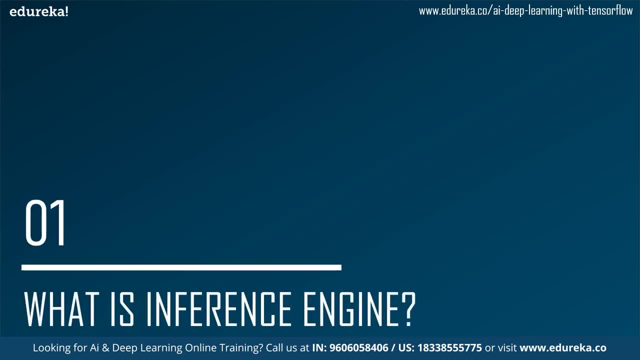 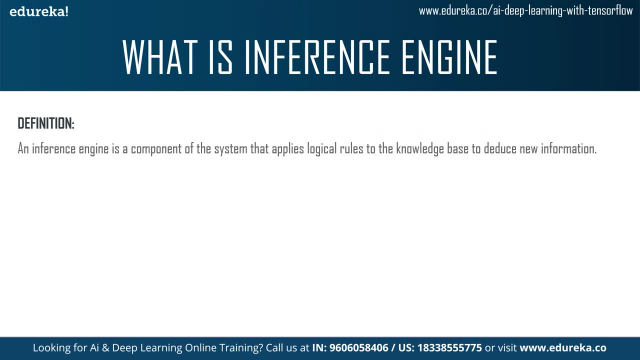 of what these concepts are. By definition, an inference engine is a component of a system that applies logical rules to the knowledge base to deduce new information. This means that you have a collection of data, or what you call a knowledge base, and you find information that you want by applying. 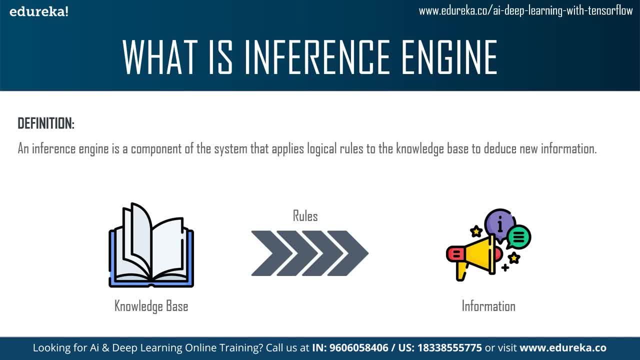 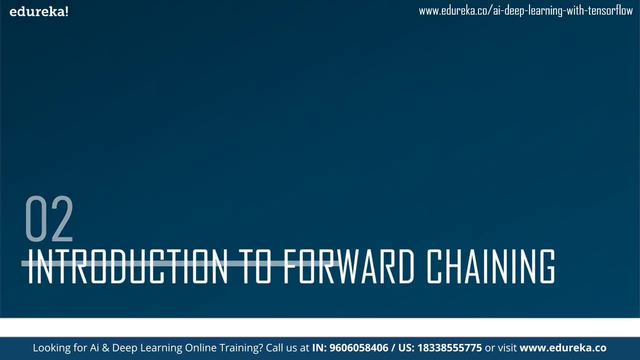 rules to it. Now, there are mainly two types of inferences, As you can guess. it is forwards chaining and backwards chaining. So let us get started with forwards chaining. By definition, forwards chaining is a form of inference. It is a form of inference that allows you. 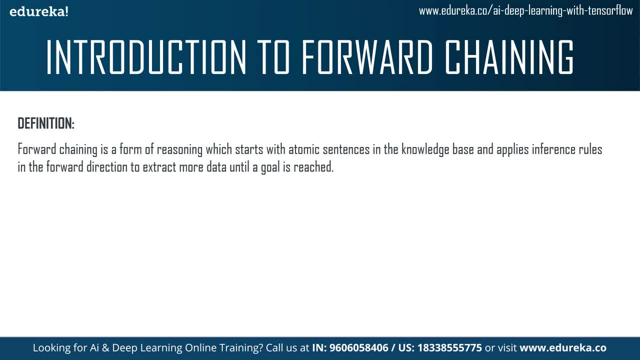 to deduce new information. It is a form of reasoning which starts from atomic sentences in the knowledge base and applies inference rules in the forward direction to extract more data until a goal is reached. So you reach a goal by analyzing and inferencing upon your knowledge base. Now how do you process? 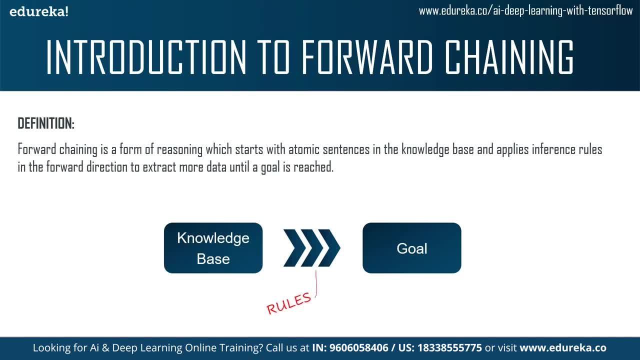 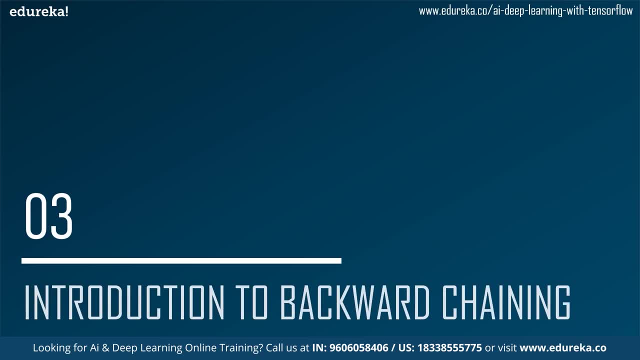 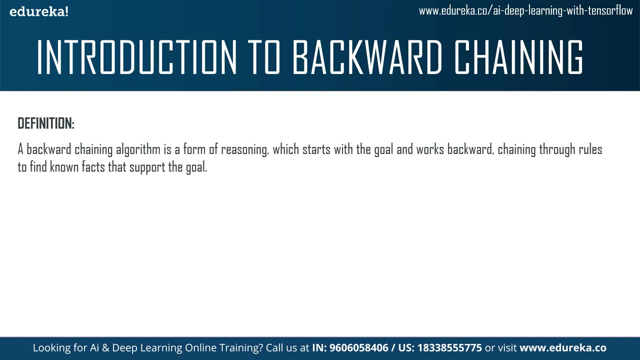 that data. You do this by applying rules, And that's all you need to know about forwards chaining. It's that simple. After this, you have backwards chaining Over here. what you do is start from the goal and then apply rules in such a way that you get to the problem. As a definition, you can. 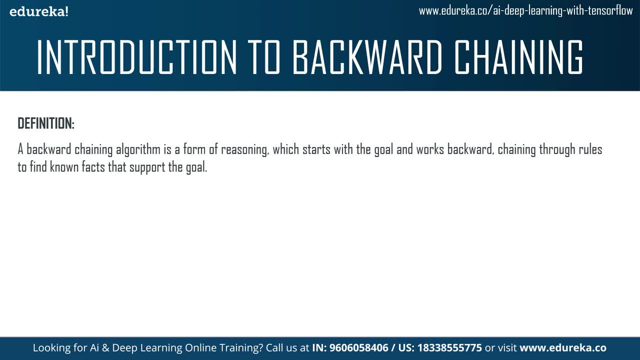 refer to this. A backwards chaining algorithm is a form of reasoning which starts from the goal and works backwards, chaining through the rules to find known facts that support the goal. So this is pretty much the reverse of what you saw in forwards chaining Over.